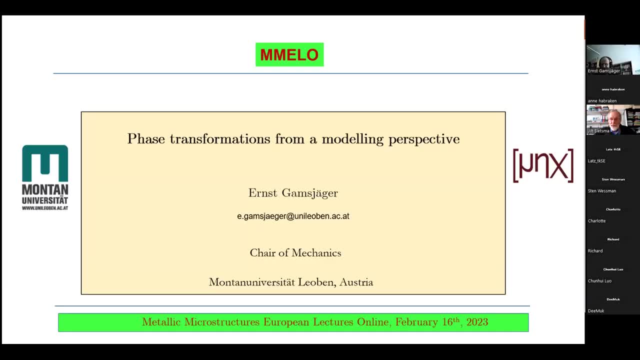 And welcome all the attendants, but especially Professor Ernst Kampschäger, who will be the speaker of today. He is Associate Professor at the Chair of Mechanics at the Montaigne University in Leeuwin in Austria. He's been there since 2010 in this position. 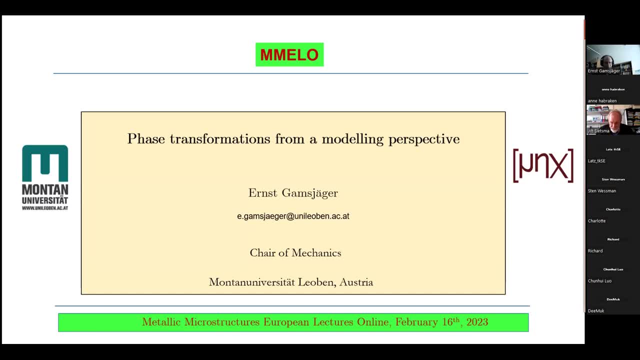 And his research fits perfectly well in this series of lectures about thermodynamics, phase transformations, micro-mechanics of materials, but exactly the things we want to look at. He received the prestigious Maasing Memorial Prize in 2010.. That's the prize of the Deutsche Gesellschaft für Materialkunde. 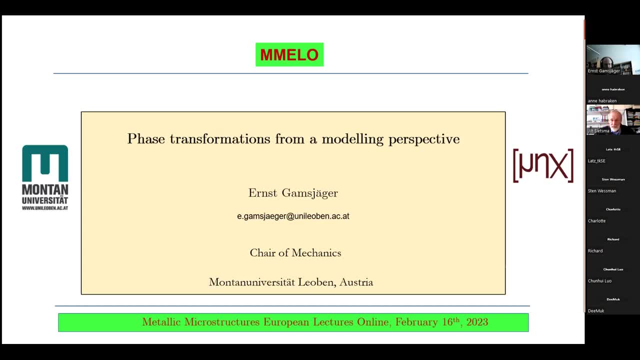 As I said, his research. the topic fits perfectly well in this series, So I'd like to give him the words, with the title for his presentation being Phase Transformations from a Modelling Perspective. Ernst, please, The floor is yours. Thank you, Professor Sietzmer. 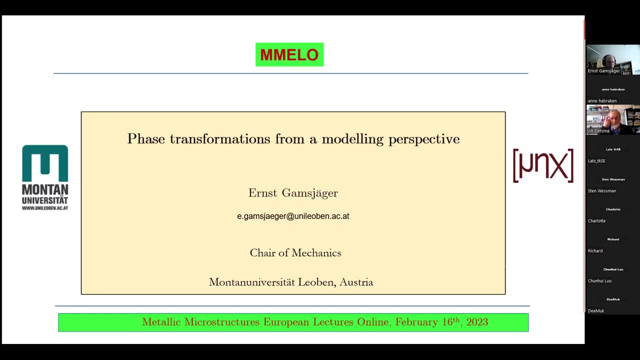 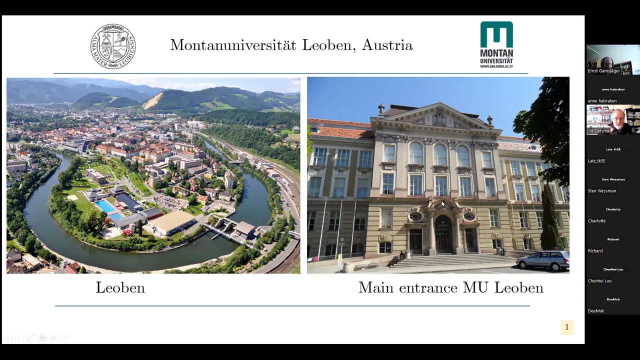 Thank you, Yield, for this very kind introduction. And yeah, I will talk about phase transformation from a modelling perspective. And please allow me to show the university town, beautiful town, Leeuwin, in Austria. And here is the entrance, main entrance. 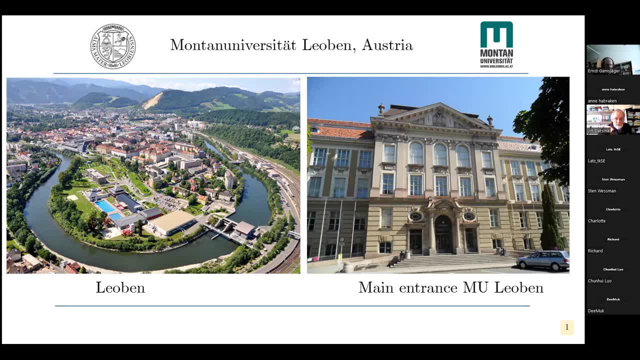 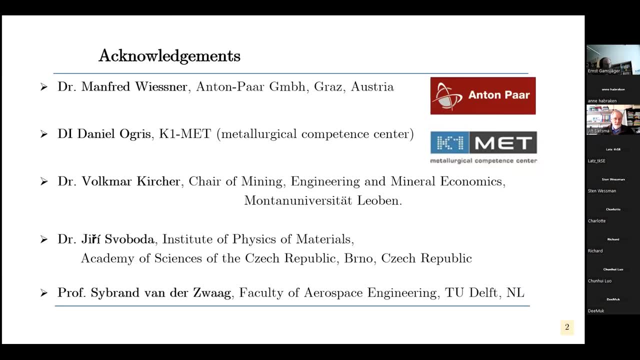 And here is the entrance of our university, now a little bit more than 180 years old And, yeah, started in a mining tradition. And I also want to acknowledge my co-workers, Dr Manfred Wiesner from Anton Bar Company and my PhD student, Daniel Ogris. 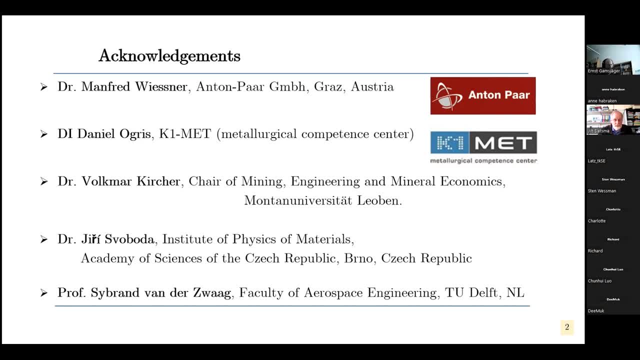 And the experiments with the high-temperature laser confocal microscope did. Dr Volkmar Kircher and Dr Jerzy Svoboda and Professor Sipan van der Swaag are also long-time scientific companions, I would say, And I acknowledge this very much. 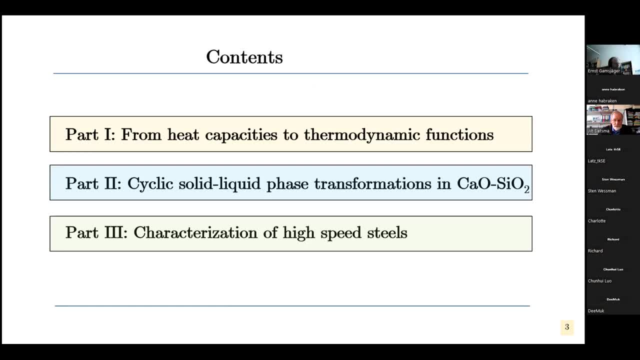 So my talk will be in three parts. First part is thermodynamics, from heat capacities to thermodynamic functions, And then we switch to thermodynamics of irreversible processes, cyclic solid-liquid phase transformations. And finally, I want to characterize high-speed steels. 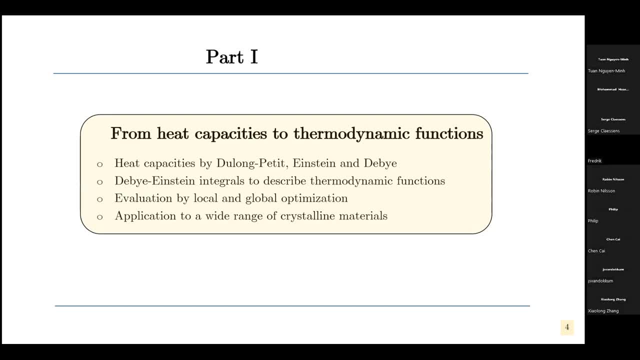 Yeah, from heat capacity to thermodynamic functions, the heat capacity models. Oh, please mute yourself. Please mute yourself, or you can also do it. Okay, Yeah, the heat capacities. First, I want to introduce the law of Toulon-Petit and Einstein and Debye. 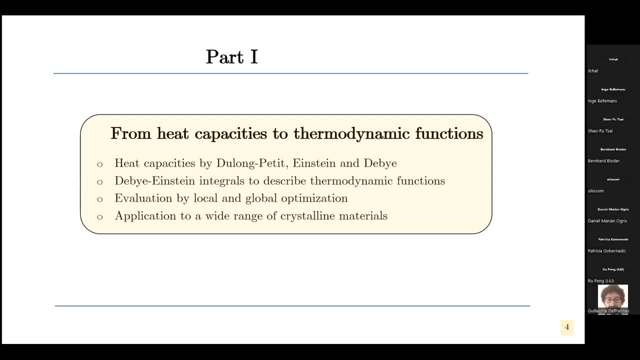 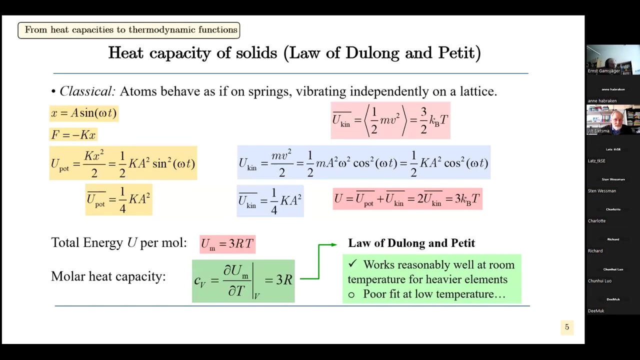 And with Debye-Einstein integrals we can describe all thermodynamic functions. And these fitting models will be evaluated by a local and global optimization tool. And it can be applied to a wide range of crystalline materials. So to introduce the capacities, classically one thinks of atoms which behave as if on springs. 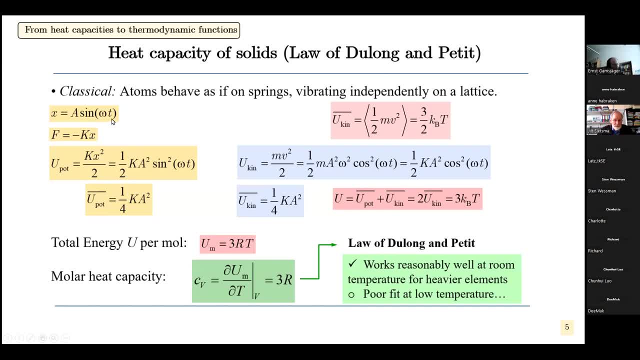 And then the elongation is a sine function of time And the force is proportional to the elongation, And one can calculate the potential energy, which is then a function of time, And also the mean potential energy, And the derivative of the elongation is the velocity. 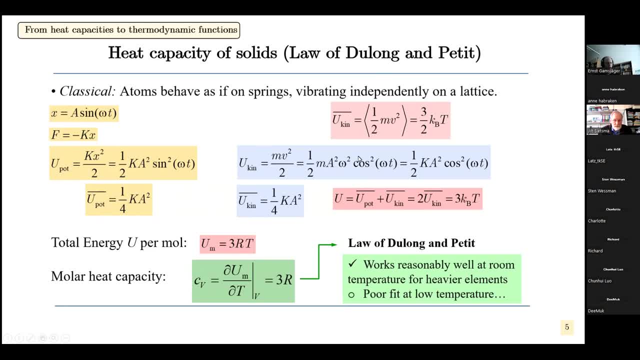 And therefore one can calculate the kinetic energy as a function of time And again also the mean kinetic energy And the sum of the two, the potential and the kinetic energy, which appear to be the same, gives the whole energy of the atomic spring and the mean value of the. 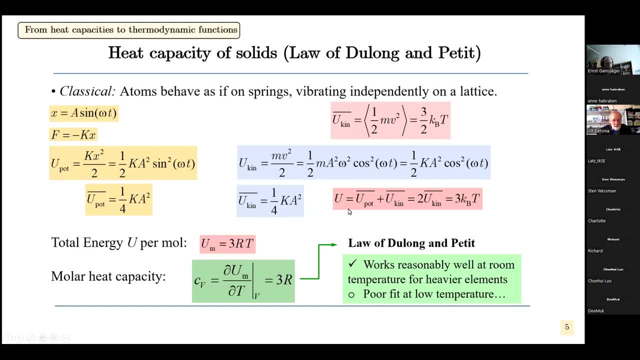 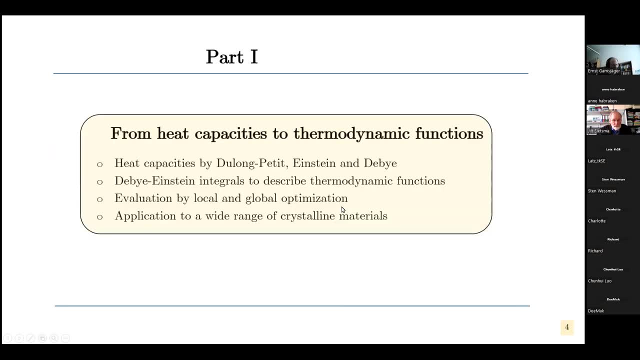 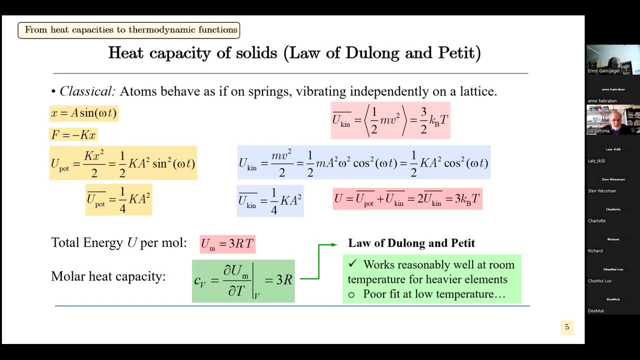 kinetic energy, we know, is related to temperature, so we can relate the energy- sorry, we can relate the energy of the system to the temperature, and for one atom it's three times the boltzmann constant times the temperature, and for one mole it's then three times the gas. 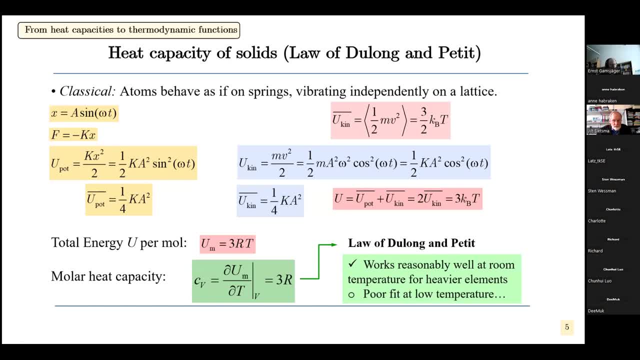 constant times temperature, and one can easily calculate the heat capacity which is then at constant. once for two atoms, зive and the integral of d5, sempre order in r stood z and for the floating motor and a constant of 2 times the current energy in the center of the mass and 3 percent of the sample taken from both the operator and j i �ories to be the constant. 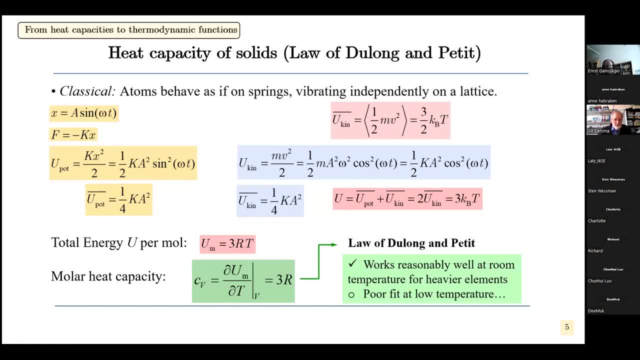 And one can easily calculate the heat capacity, which is then at constant. once for two atoms, Mach and one California volume 3r, which is the law of too-long-and-petit, And this turned out to work reasonably well at room temperature for heavier elements. 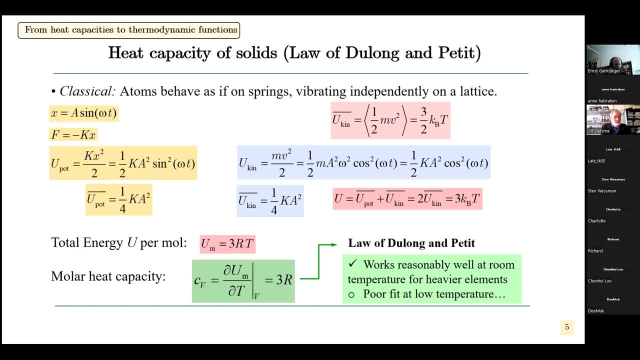 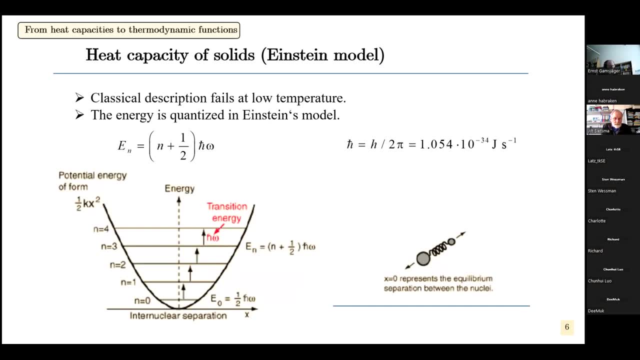 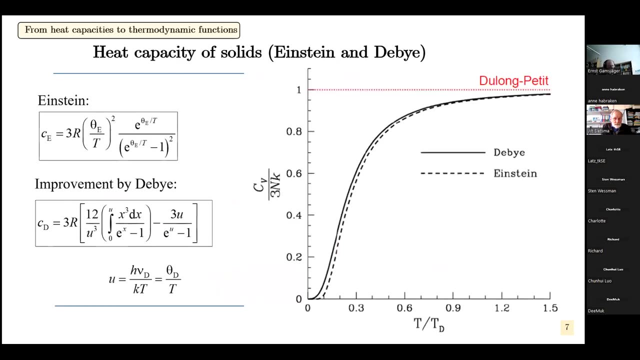 but is a really pure fit at low temperatures, And therefore Einstein came up that the energy is quantized. So we have a quantum atomic spring And with this model the experimental data fitted much better And there has been even an improvement by Debye, who thought that there is not only 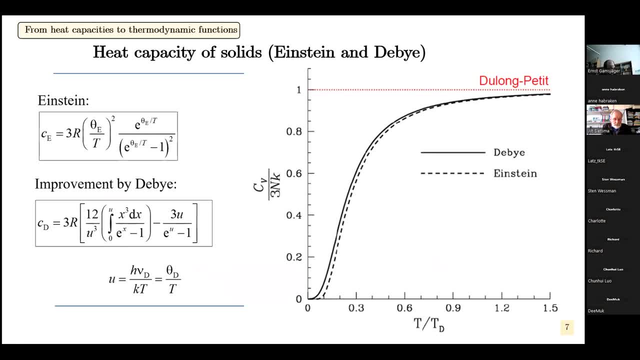 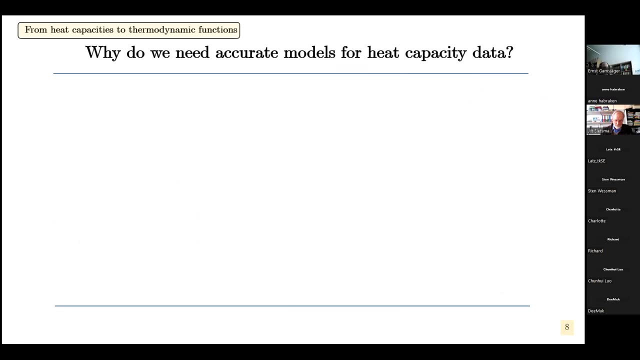 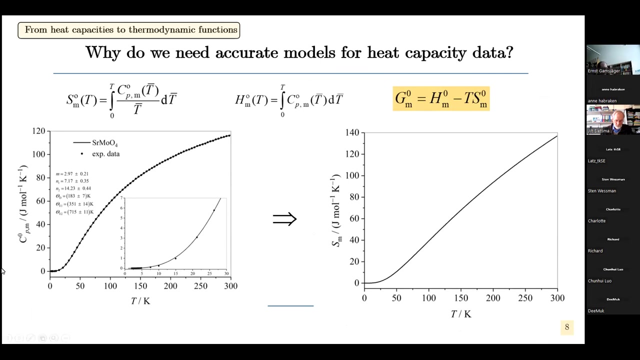 one atomic spring, but they are all connected in the crystal lattice, And this then gives a real good description of the ultra-low temperature range of the heat capacity. And so why do we need it? We need accurate models for heat capacity. So nowadays we have very precise calorimetric measurements for the heat capacity, down to 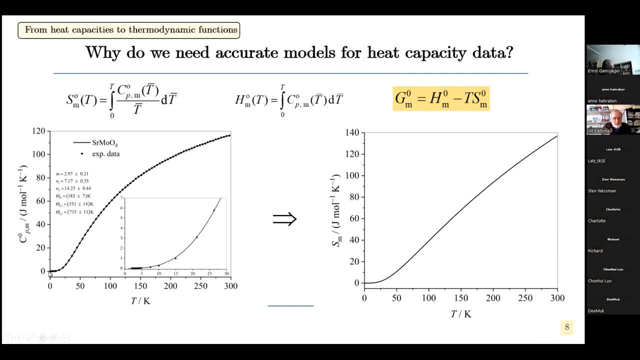 very low temperatures And we want to describe that here, for example, with this six-parameter fit with some constants and the Debye and the Einstein temperature, And from that we can calculate all other thermodynamic functions like the entropy, like the entropy and the Gibbs energy, of course. 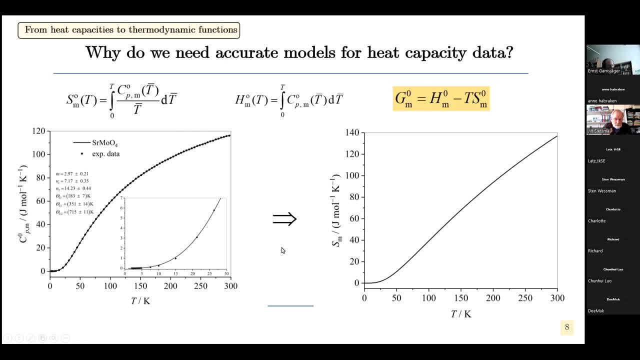 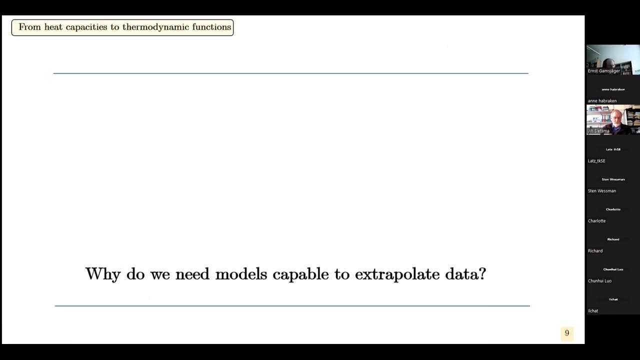 And then, with this accurate model, we can put all this experimental data into this six constants, of course, And then we can calculate all the other functions. And what is also good with this Debye-Einstein approach is that it's possible to extrapolate. 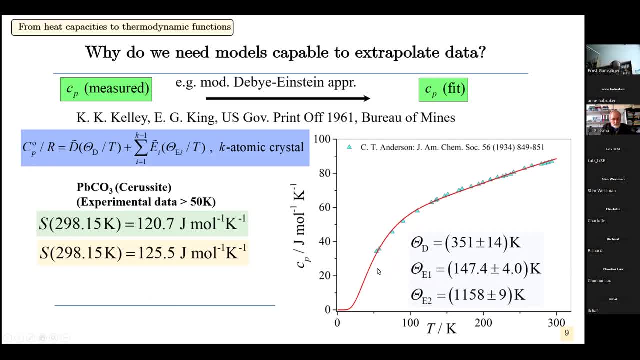 data. Very often we don't have low, ultra-low temperature data but all the measurements there we can only there the people could only measure down to 50 Kelvin, And then this Debye-Einstein approach allows to extrapolate data. 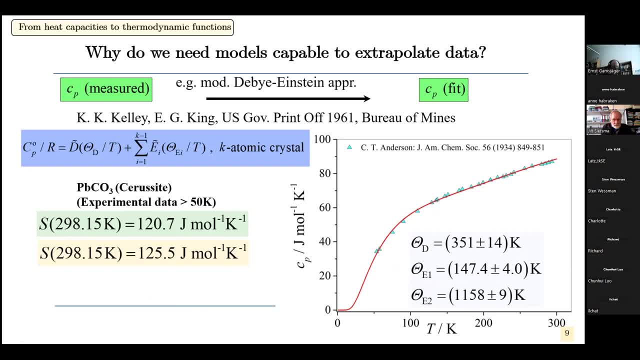 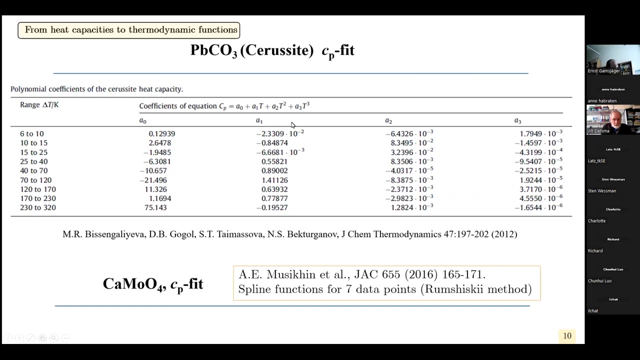 And then this Debye-Einstein approach allows to extrapolate the data in a useful way And then to get all thermodynamic functions at room temperature, for example- And yeah, this was the approach by Kelly and King- And then the precisely measured heat capacities are measured by are modeled by various polynomials. 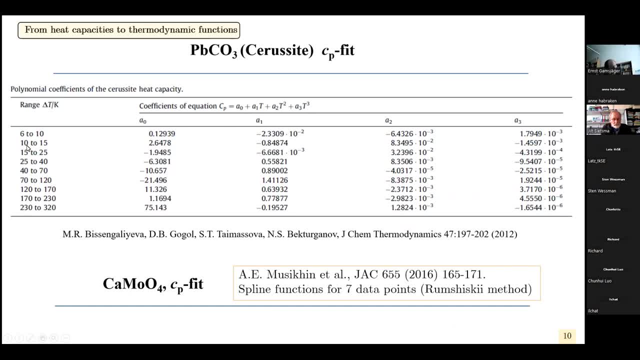 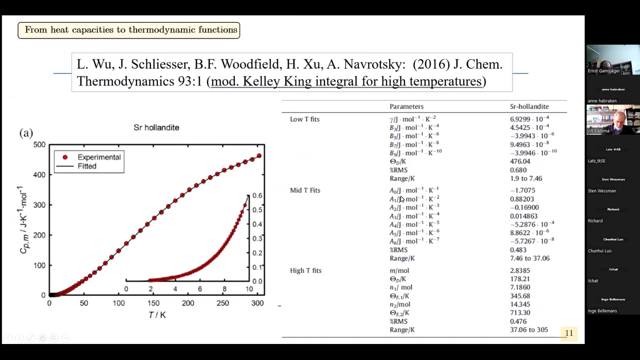 Here you can see, for example, in the temperature range between 6 and 10 Kelvin there are already four coefficients, And then there are a lot more, And sometimes this leads to overfitting. And here is another example where we have low temperature fits, mid temperature fits. 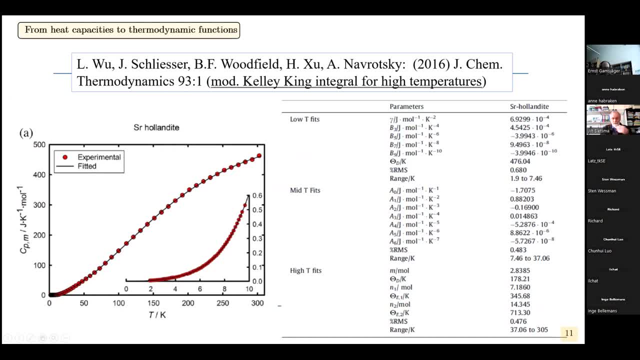 and high temperature fits. So high temperature begins here at 37 K And also the temperature ranges are quite arbitrary, so 1.9 to 7.46.. But the high temperature fit here, used here. we use that for the whole range. 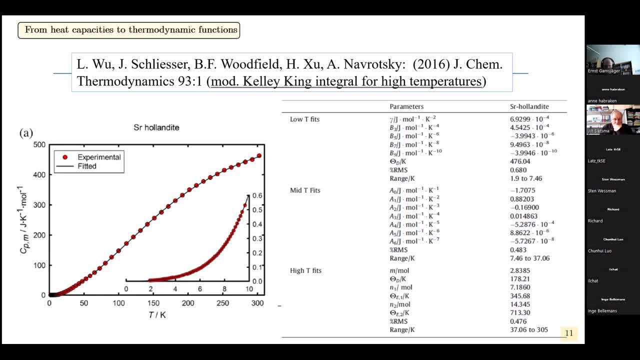 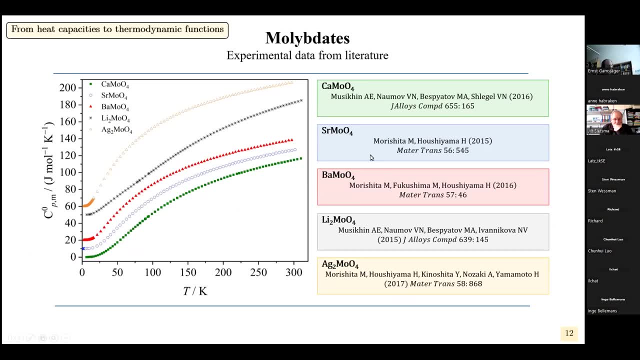 And I think we could show that. But for many materials this is really sufficient, And so this is what I want to show you here with the molybdates. These are the experimental data, And of course the heat capacity have all to start at 0 Kelvin, at 0.. 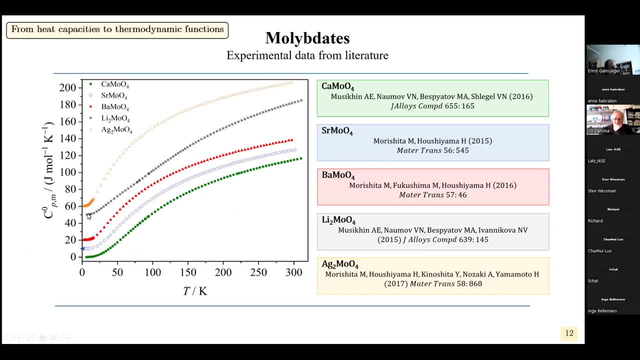 But in order for you to see better the measurements, I shifted the strontium molybdate heat capacity by 10 Kelvin, And I also shifted the strontium molybdate by 20 Kelvin And lithium molybdate by 50.. 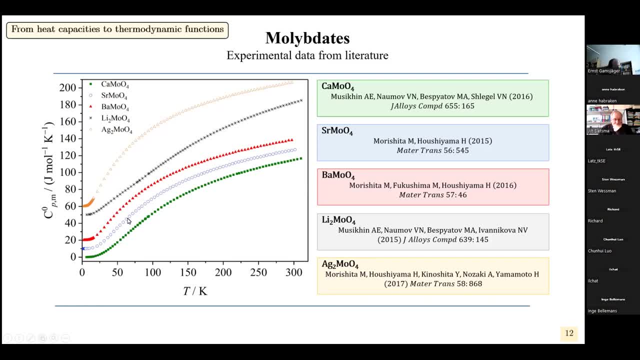 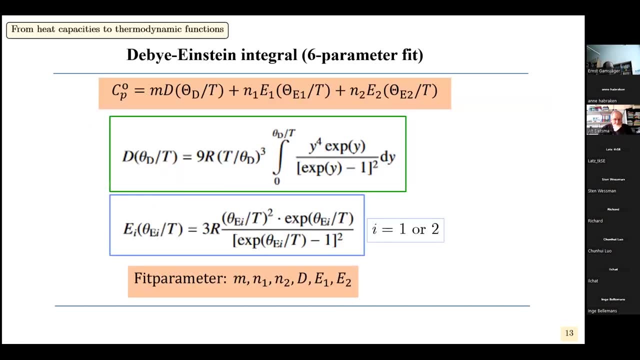 And silver molybdate by 60.. And here you see the experimental data And with this fit function. so three pre-factors And the temperature, which is here the fitting parameter, one Einstein function and the second Einstein function. all these molybdates and many minerals. 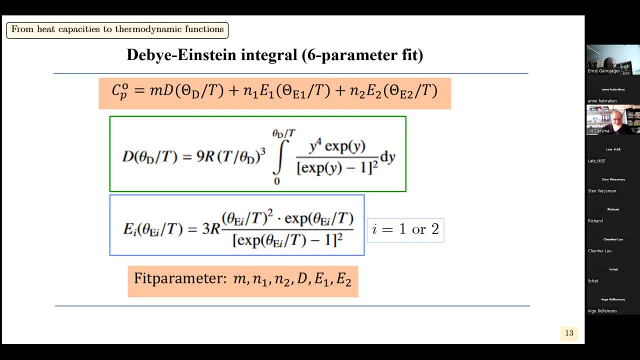 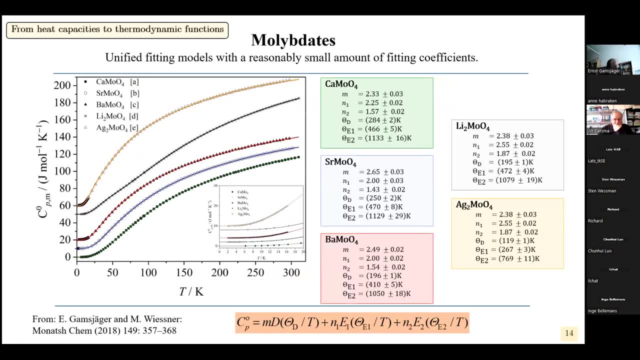 can be. the thermodynamic data can be described very well between 0 Kelvin and room temperature, And here you can see this for the molybdates. and this was done by a local fitting procedure. so this square fitting Levenberg-Marquardt with the help of Origin. 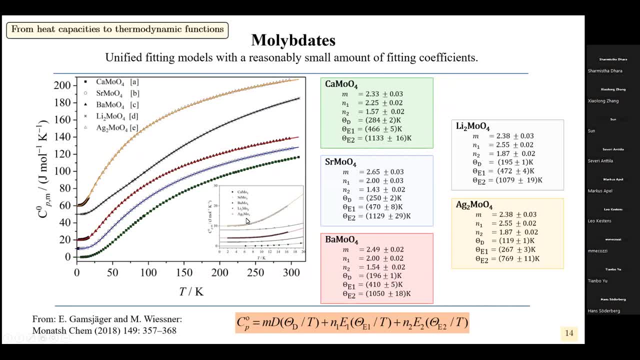 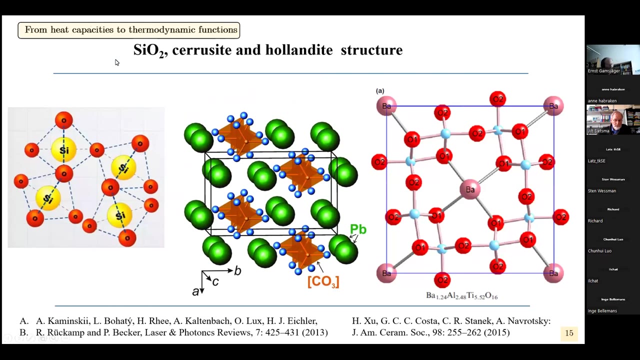 and you can see also here in this insert that also for the very low temperatures, from 0 to 20 K, the fit are quite good. This is not always the case, but for molybdates it worked very well. And here we have different minerals, so quartz and 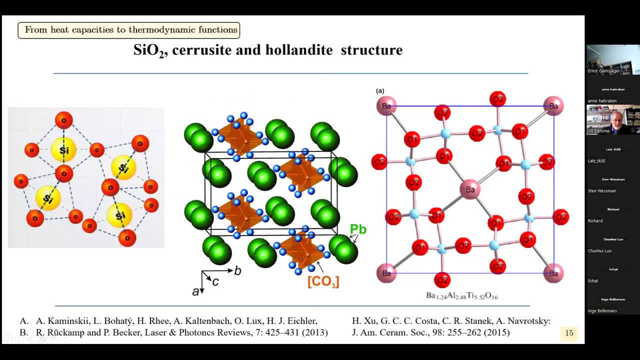 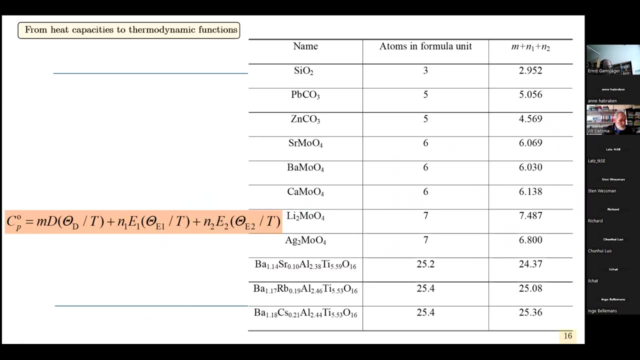 cirrusite and hollandite structures. Hollandite they use, for example, to immobilize high risk nuclear waste, and so they want to know the thermodynamic properties of these materials. and for all these materials we can see that yeah, one. we tried to fit this data and by the Levenberg-Marquardt fit. 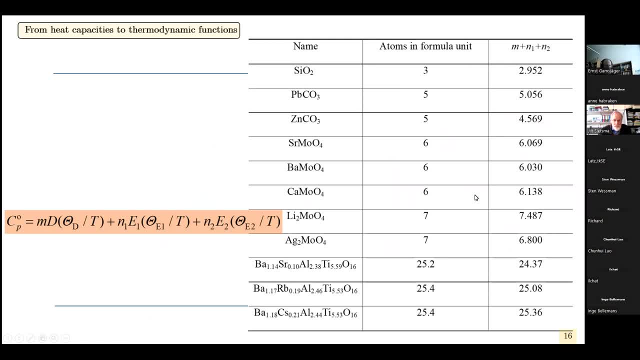 algorithms, And here you can see the atoms in the formula unit and, from the theory of course, the sum of M plus N, 1 plus and 2, this where the three factors has to be the same as the number of atoms in the formula unit and but. 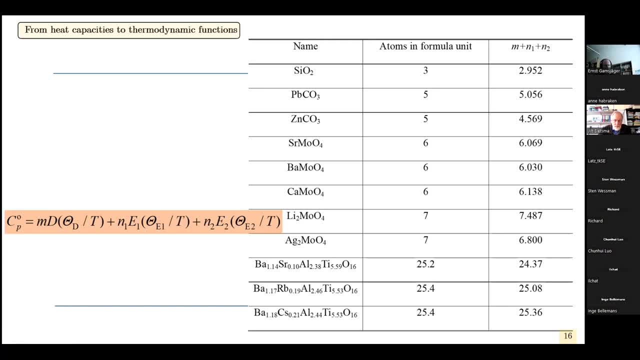 the Levenberg-marquardt quad algorithm does not know anything about it, of course, and, yeah, it approximates the theoretical value, i think, in many cases quite well. so here, here is maybe a bit deviation, but this works quite well. so it's a empiric approach, but with, i think, which makes a physical sense. 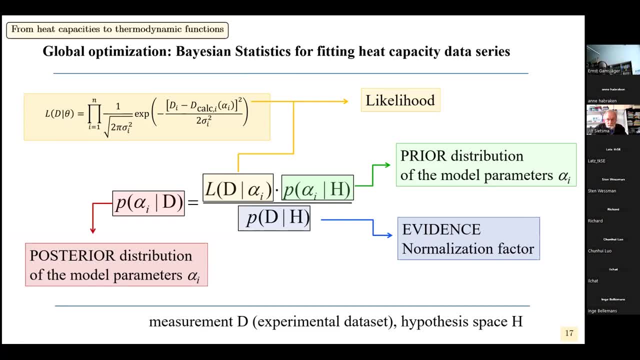 and now we wanted to test this local optimization routine with with a global optimization by bayesian statistics. and there we start with a prior distribution, with some assumptions, and then from the measurements and the calculations one can calculate the likelihood. and this is done by a monte carlo markov chain algorithms in order to get the best posterior. 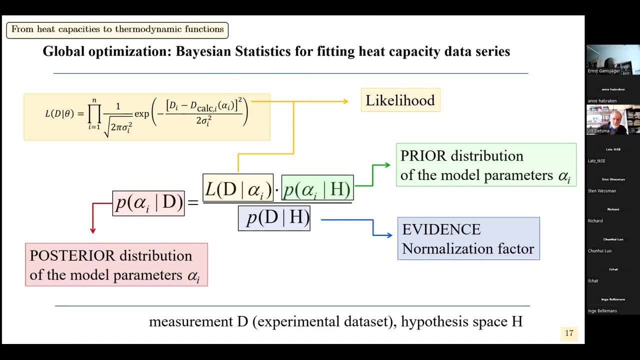 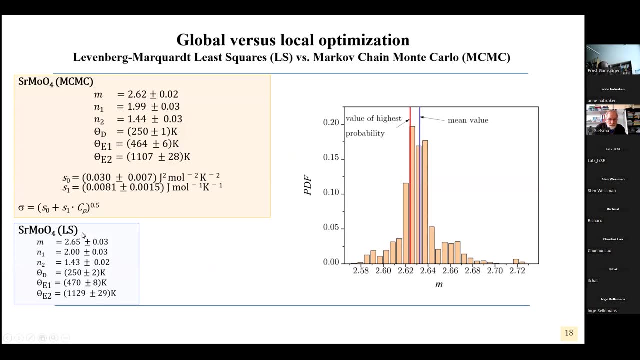 distribution and the model parameters, the three pre-factors and the divide temperature and the two einstein temperatures. and here is the comparison between least square method and the monte carlo markov chain algorithms. and the model parameters, the three pre-factors and the divide temperature and the divide temperature. 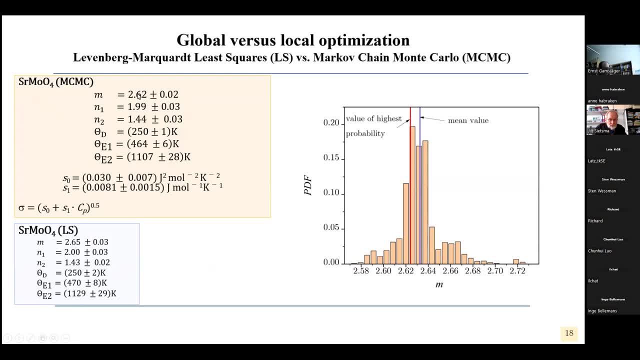 method and you can see that the mean value and also the uncertainty really in the same range. and here with the global optimization routine we also calculated something like: yeah, it's a standard deviation, so uncertainty, the uncertainty range we calculated here more or less. and yeah, with the global optimization we always get a probability density function. 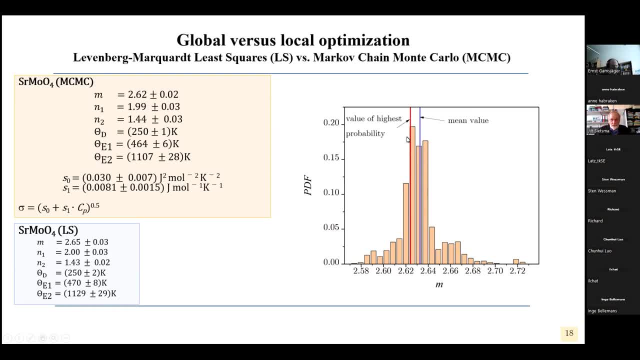 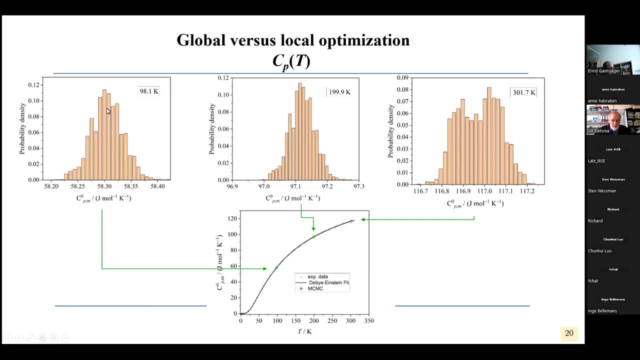 and we can calculate the mean value and the value of the highest probability. and here, for different temperatures, we can see the, the cp values, and the mean value is always practically on the curve. we also got the mean value, so the cp values are very important for the model optimization. without an optimization, the demand value is創造. 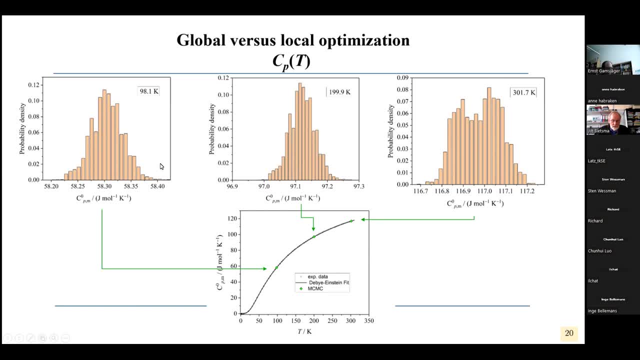 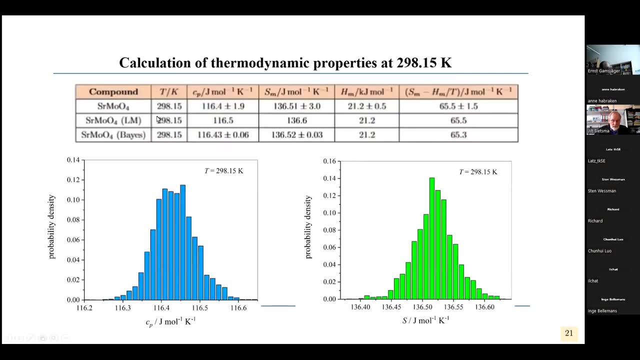 we also got from the local optimization routine and with that one can now calculate with Levenberg-Marquardt or with bias all the CP values of course and the entropy and enthalpy and the Planck-Massieu function, sort of Gibbs energy, and yeah, they are really, really very. 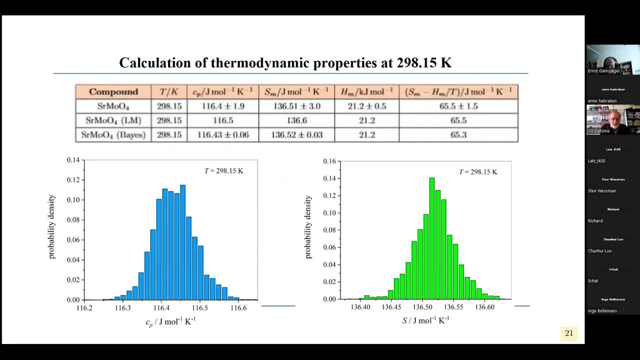 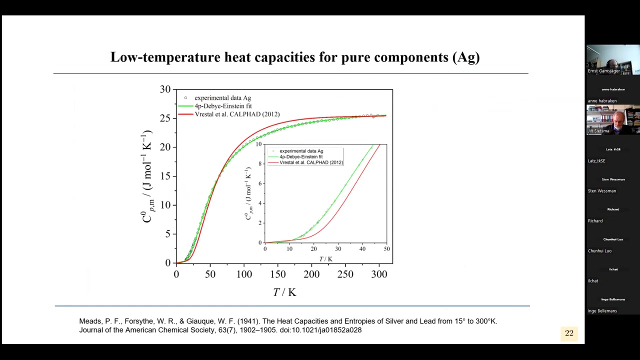 similar. so I would like to advocate this six parameter approach, always to use for materials below room temperature to describe the thermodynamic functions. and here we tried it for pure elements. so for unaries, here is silver and an older approach. so this car for third generation gives this fit and of course the debye is makes, makes. 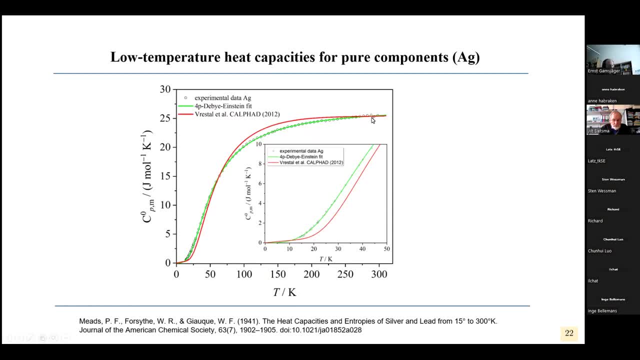 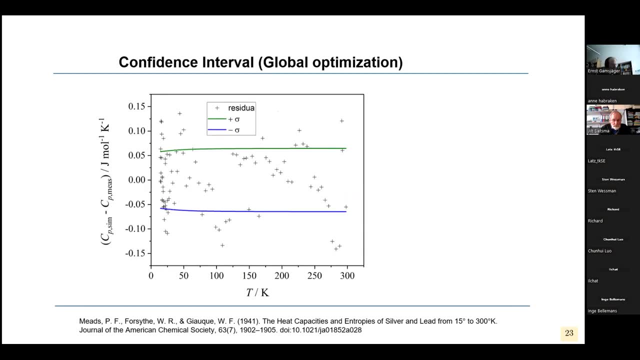 the fit, then a bit better, at least until room temperature. and, and here what we also calculated, as I said, is this confidence interval, here plus sigma and minus sigma, and here plotted the residuals versus temperature. yeah, and I think this: it works quite well to approximate heat capacity by these debye-Einstein functions. 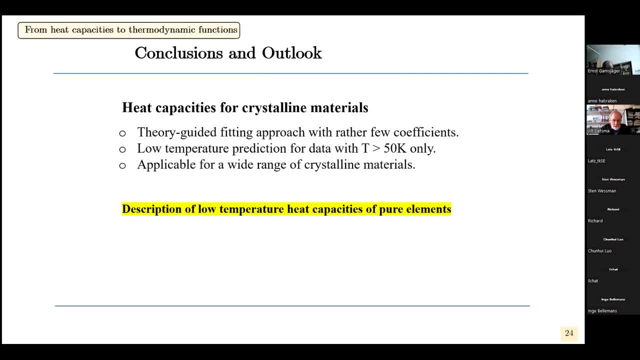 and yeah, to conclude this first part, this was very interesting and I hope that you enjoyed it. It was a theory-guided fitting approach with rather few fit coefficients. it it is possible to predict the heat capacities when we have only experimental data for temperature higher than 50 K, and it's applicable for a wide range of crystalline materials, essentially when 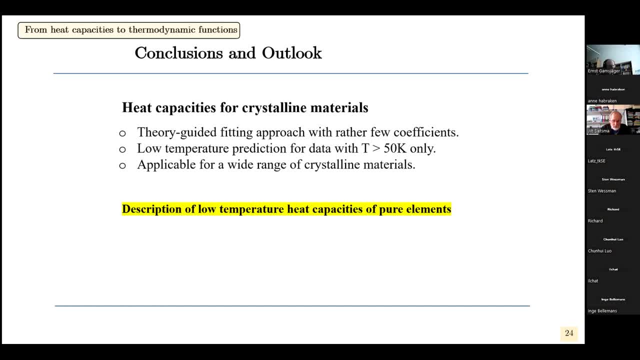 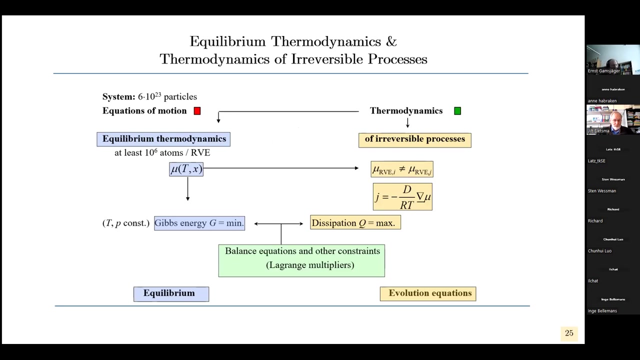 you have no phase transformations in that range. it's easy, and I think that pure elements and hand members, unaries, should be described in a sort of standard way by by such an approach. so and now we switch from equilibrium thermodynamics to the thermodynamics of irreversible processes. but- and yeah, we know why do we use thermal? energy and we know why we use heat capacity. we can't use thermal energy. we can't use thermal energy. but think about the thermal process, right? i mean heat capacity. that we're talking. we're talking about the problem here. we're not. we're not talking about heat capacity, we're. 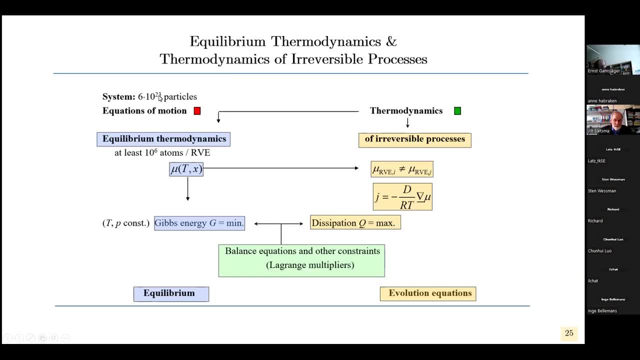 use thermodynamics because when we have 6 times 10 to the power of 23 particles, it's not possible to calculate all the equations of motions. And so now we look at equilibrium thermodynamics, for in one representative volume element can we calculate a temperature and the chemical potential. 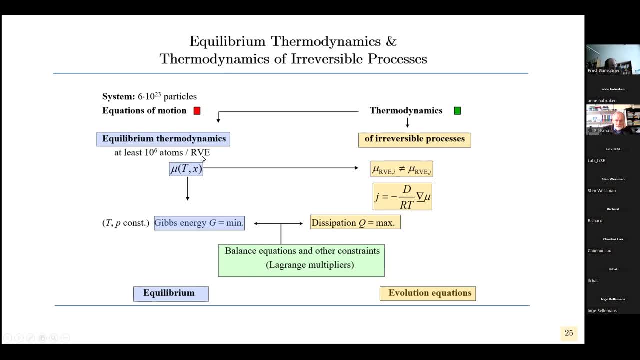 when we have 10 to the power of 6 atoms inside this RVE at least, And then we can calculate all these properties locally and finally minimize the system here. When T and P is constant we minimize the Gibbs energy But two neighboring RVEs volume elements. 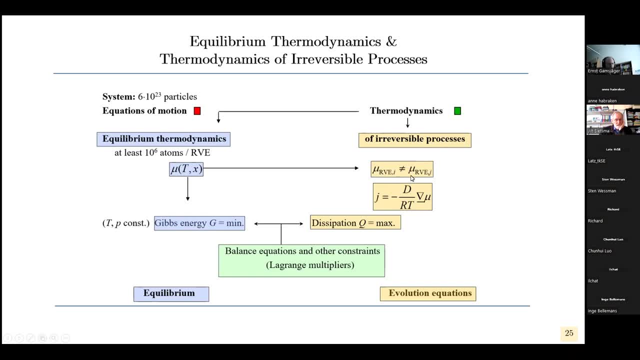 they can have a different Chemical potential, And then we could assume that the difference in this chemical potential is proportional, for example, to the flux of the components. And then we take into account irreversible processes. in the framework of this local equilibrium And with maximizing the dissipation, 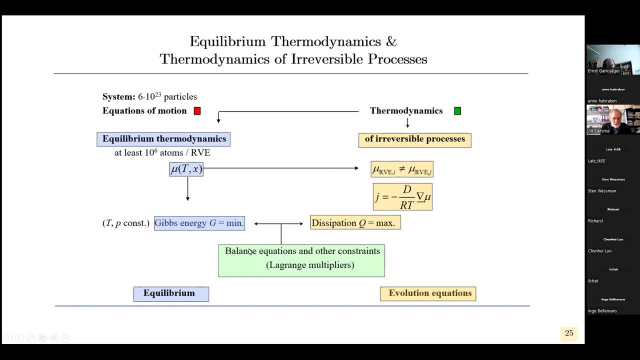 we would have a very linear distribution And, using balance equations and possible other constraints, we come to the evolution equation in the sense of irreversible processes, Or we come to the equilibrium, when we simply minimize the Gibbs energy And the evolution equations, of course, 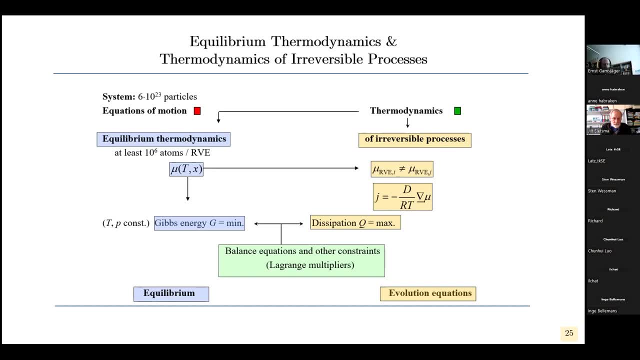 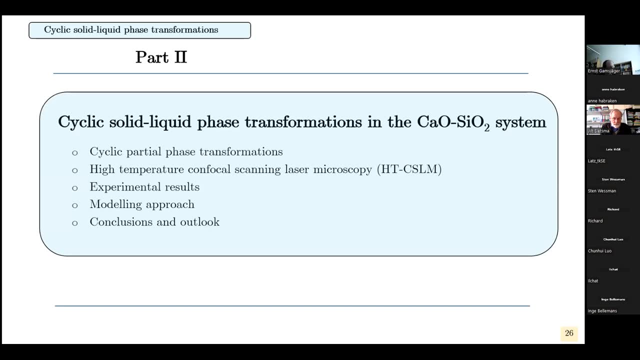 finally leads to a steady state Or to The the equilibrium also. so now to the irreversible processes part. we want to look at cyclic solid liquid phase transformation in the CAO CO2 system. and first I want to say what are cyclic partial phase transformations? 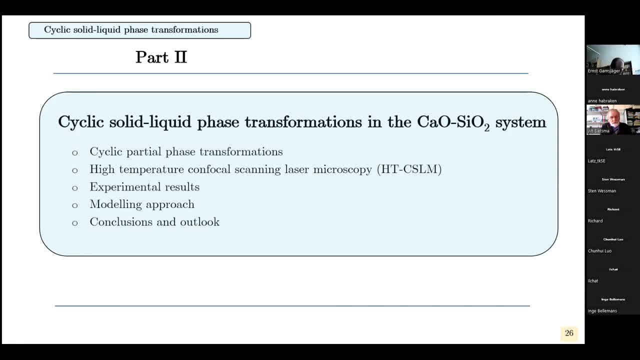 this was introduced by Professor van der Swaar and his co-workers, and we'll show this in a minute. as an experimental tool we have the high temperature confocus scanning laser microscope, and then we will compare the experimental results with the modeling approach, and then I will. 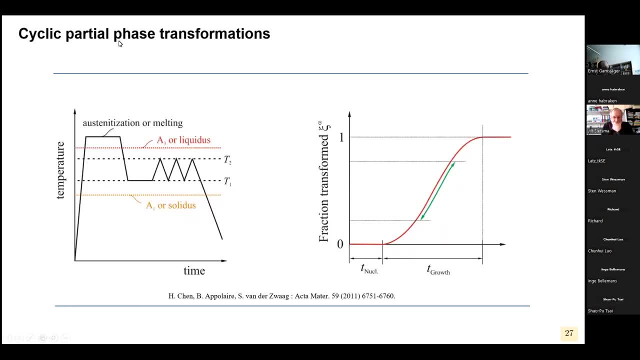 conclude this part. so what is the cyclic partial phase transformation? in order to avoid nucleation processes, it's good when both phases here- the solid and the liquid phase, or the austenite and the ferrite both- are present, and when the front is migrating and the 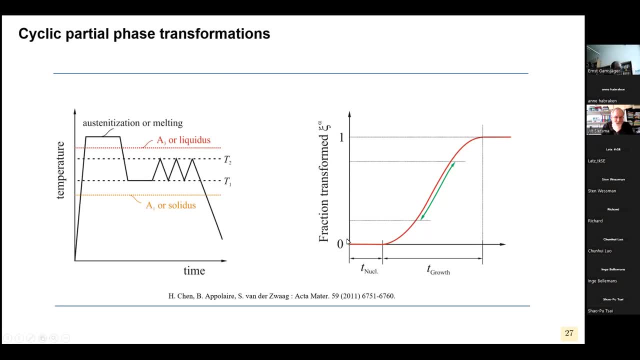 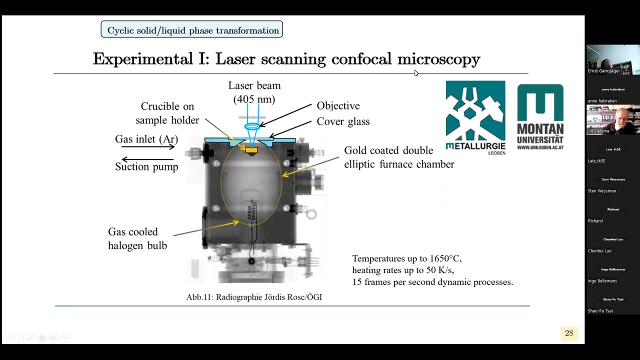 time for nucleation is not consumed. and in order to achieve this one has to cycle between in the two phase region, or at least make sure that both phases are always present. and yeah, and we did the experiments with this laser con focal microscope there, use in the middle, here you see. 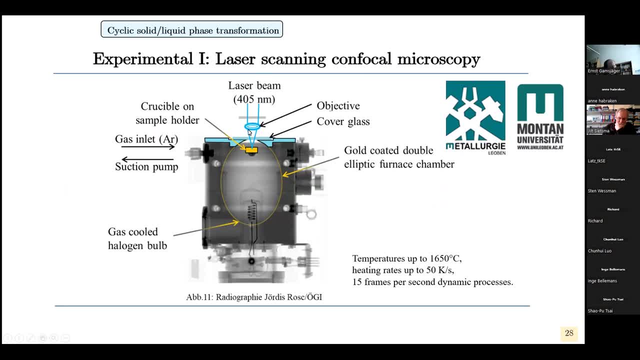 this gold coated. it's an ellipsoidal oven and here, in one focal point, there is the halogen bulb and here is the specimen which is heated very locally, locally, and the big advantage of this device is that you can go up to 1650 degrees celsius. 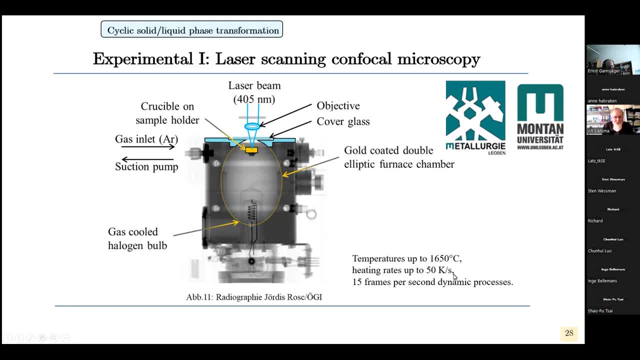 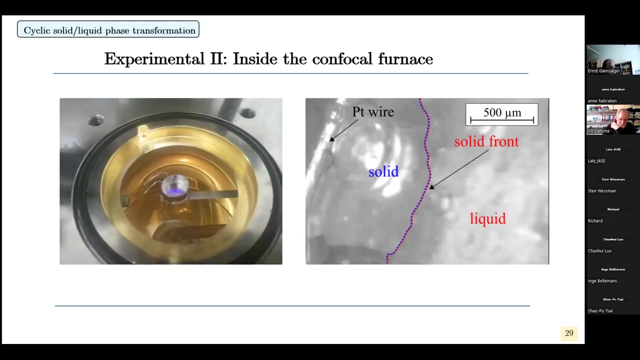 and you can get get up to very high heating rates: 50k per second, and now we can look at 50 frames per second, dynamic processes, so one. for example, one can observe martensitic needles when they are growing and and see this in situ and, but here we have the oven inside. 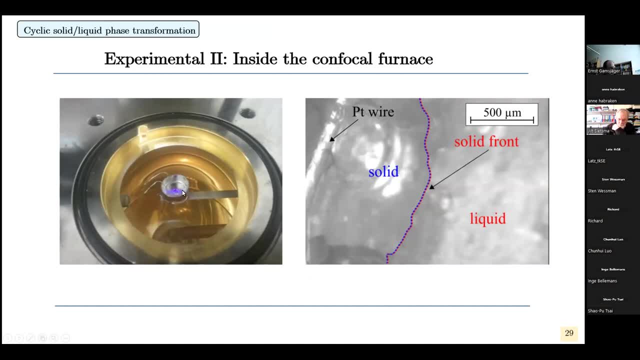 we look inside the oven, and this is the platinum crucible with the thermocouple here and there when, before the experiment starts, the powder comes in, which then will be melted at the high temperatures. and here is a platinum wire where the solid phase can nucleate. 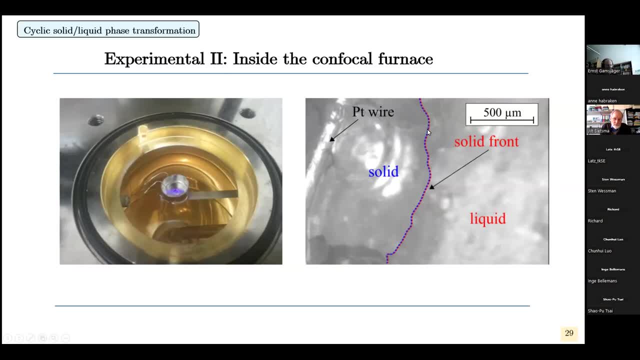 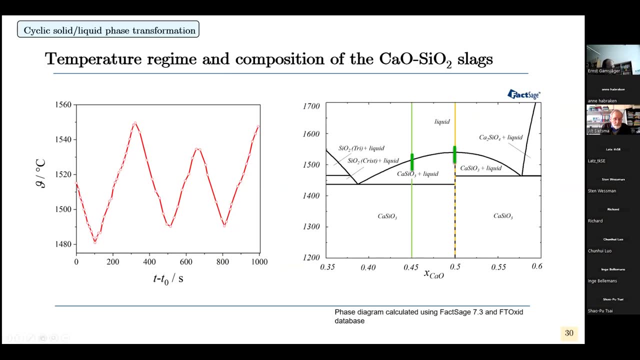 and then we have here the solid liquid front which grows or shrinks in this and here is the, the temperature treatment we had for this, and we look at two different compositions. so one is diffusion is required during melting and solidification, and the other composition here is at the maximum in the phase diagram, so the no diffusion is required. 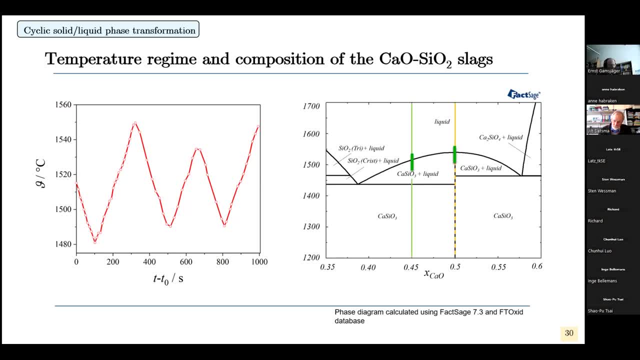 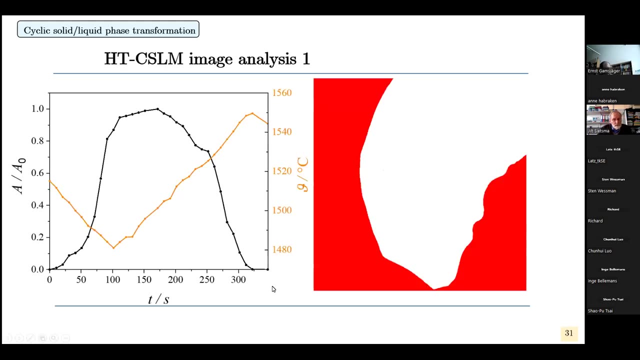 and we look at the differences between these two processes. so this is incongruent- melting and solidification- and this one is congruent- melting and solidification, and in this case solid and in this case tardive melting. and there are two ways people can munch together and not completely vogt. 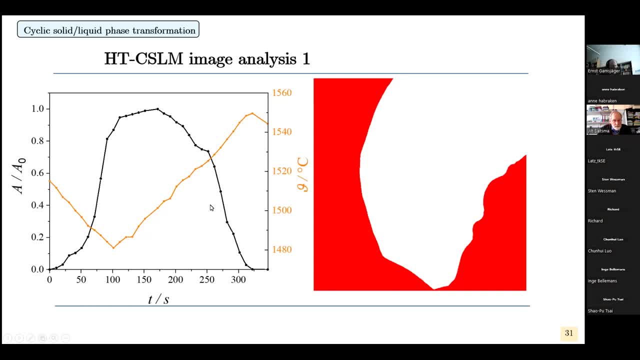 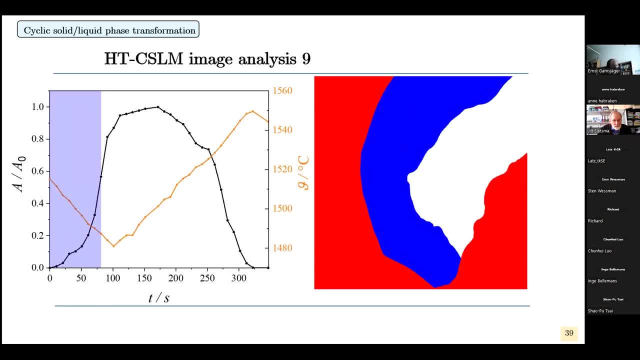 and now we can also here. we go down with the temperature and the solid phase will grow and then, when going up with the temperature again, will shrink again. i will show you that in sort of a movie. so here the time goes, grows, and now it's growing, growing, growing. 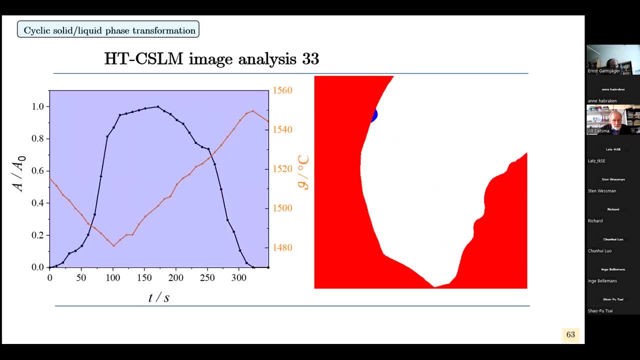 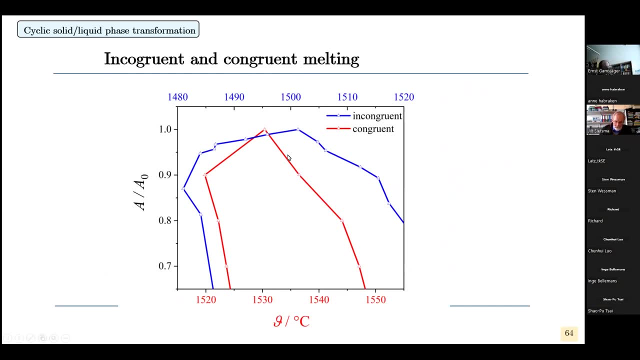 it goes back. so yeah, and we did this for, uh, incongruent and concurrent melting, solidification and melting, i have to say, and in the incongruent melting you see here sort of an inverse transformation, so the temperature goes already up and but still the solid is growing. and the same is in the congruent case. but in the congruent case, 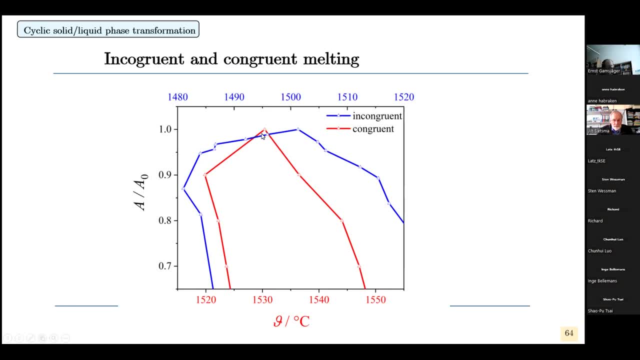 what is missing is a sort of stagnant stage. so here in this, during this time, almost nothing happens. but in the, during the congruent case, you don't have this very slow phase transformation or almost stagnant stage because the diffusion of the components is not required so that the solid liquid front advances. 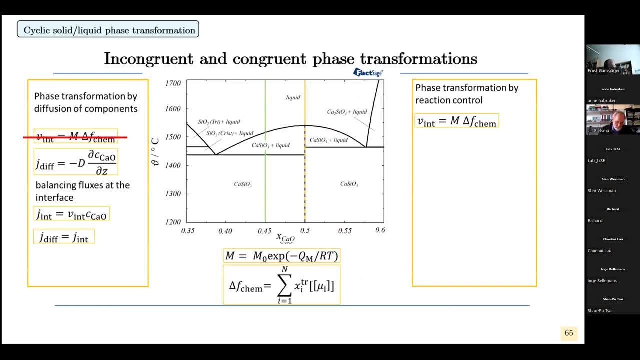 and yeah, we try to model this here with a local equilibrium, also at the interface, in case of incongruent melting. and then we have the diffusive flux, and the diffusive flux has to be equal- the interface velocity and the contrived concentration of sea air fuego here, and we have to equalize the. 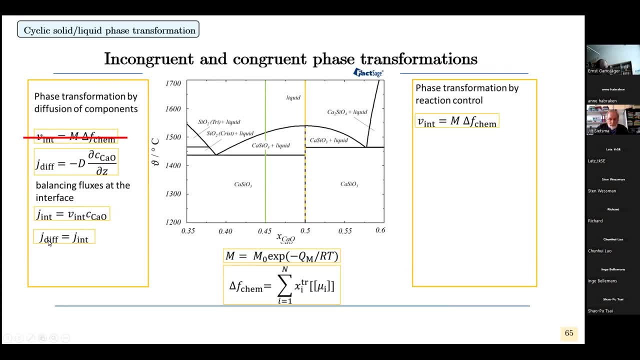 interface flux and the diffusive flux, so this is essentially connected. this is more or less the mass balance and we cannot use this linear non-equilibrium thermodynamics here with the chemical driving force and the interface velocity, because we assume local equilibrium at the interface. however, in and 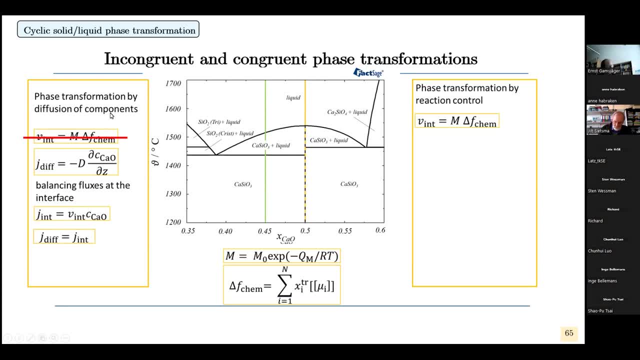 so the rate controlling process is diffusion of the components in the liquid bulk, and here, in case of congruent melting, the interface is linearly related to the chemical driving force and of course no bulk diffusion is required. so only this equation is responsible for for the velocity of the migrating interface. 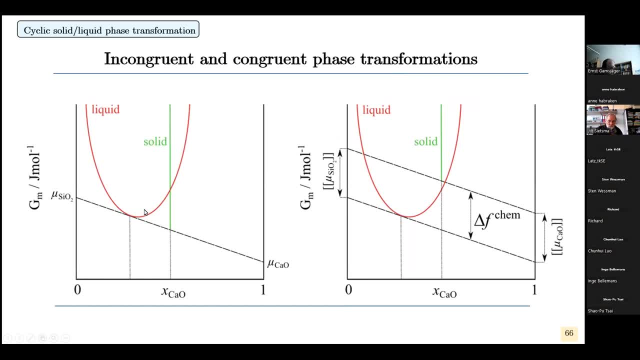 and here you can see again the ink situation at the incongruent interface. and and if we have the liquid phase and here the solid phase and the common tangent construction, and in case of the concordant phase, transformation, we have the liquid phase and the solid. 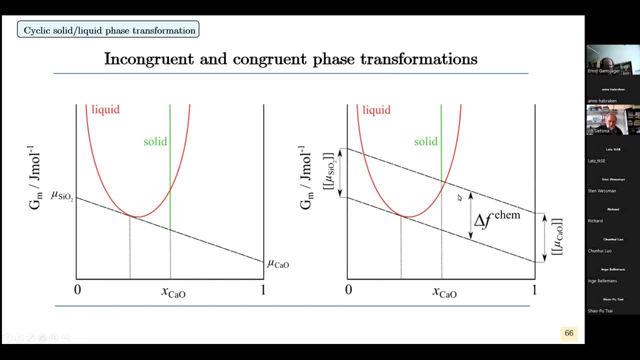 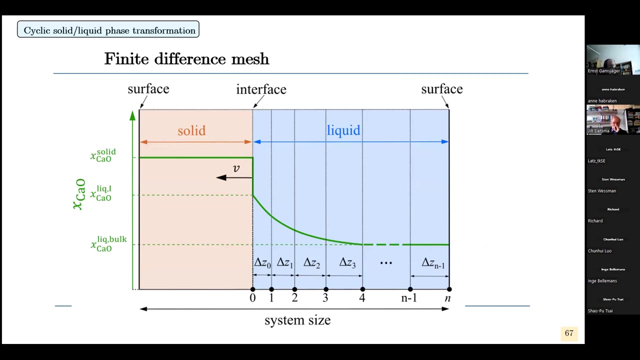 and there is a parallel tangent construction for the maximum dissipation. And these parallel tangents, they come closer and closer until they are the same when global equilibrium is reached. Here is the finite difference mesh. how we calculate it in case of incongruent melting. 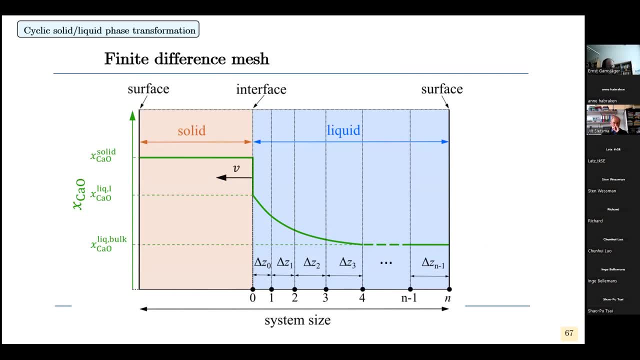 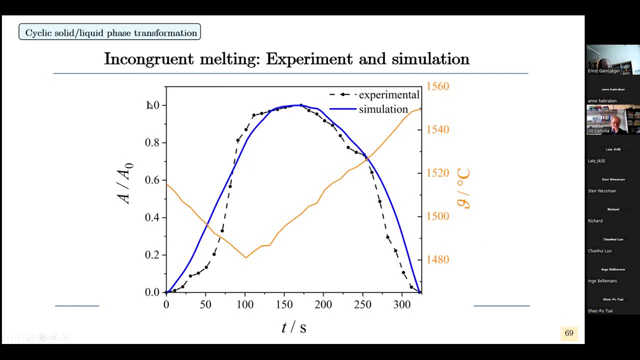 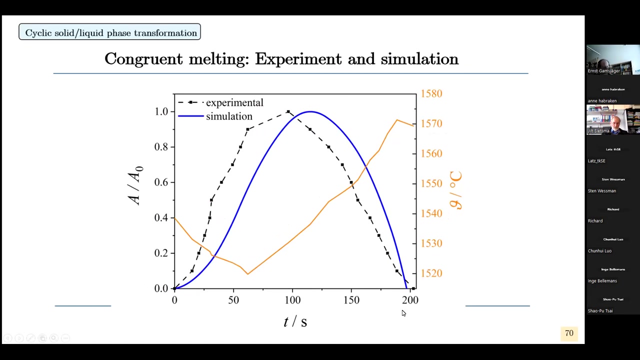 solidification, the situation And here again, difference. we have here the incongruent case, experiments and modeling. So what you see here: there is a slowdown of the phase transformation, stagnant stage, And in that case this is over a much shorter time. 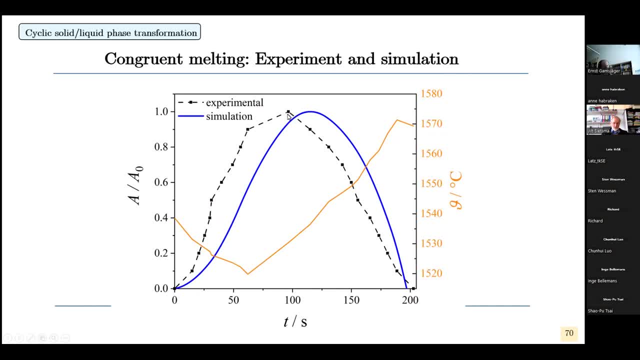 and here we have no stagnant stage. And this is the model. Maybe here the temperatures at the sample are a bit lower than written here, So there is a bit of a deviation, But I think generally both curves fit quite well Well together. 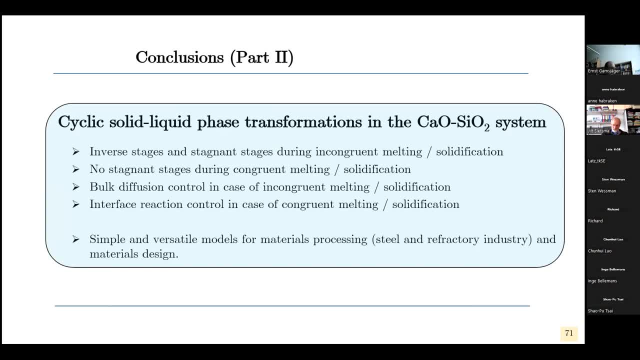 And so, as a conclusion, we can see that inverse stages and stagnant stages occur during incongruent melting and solidification, And no stagnant stages occur during incongruent melting, solidification, And with quite simple model of bulk diffusion control in case of incongruent melting. 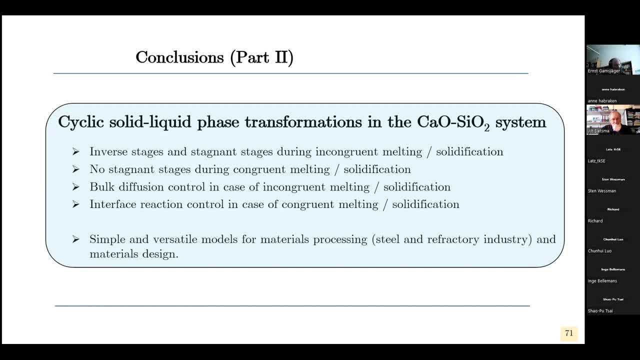 And with interface reaction control in case of congruent melting, one can model the kinetics of this phase transformation, And I think these both models are simple and versatile models for materials processing and might be applied in steel and refractory industry and can be used for materials design. 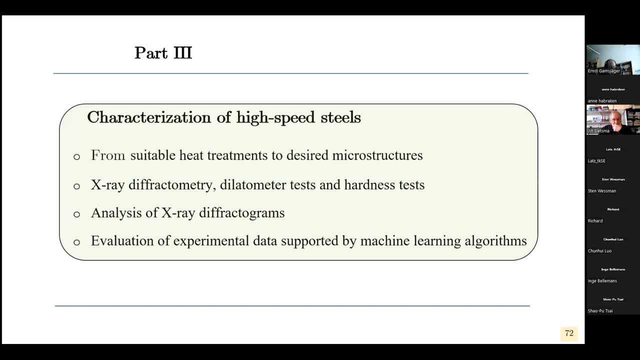 And now I would like to come to the final point, which is the material processing. And now I would like to come to the final point, which is the material processing. And now I would like to come to the final point, which is the. 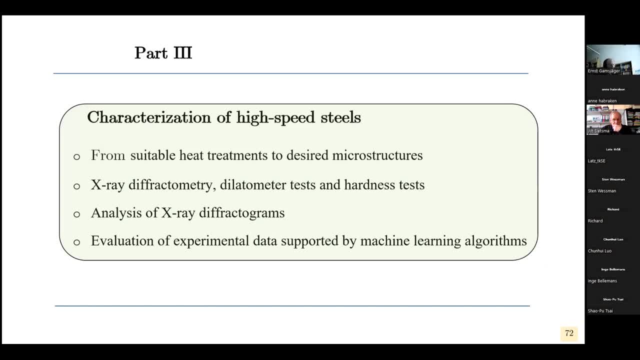 material processing. And now I would like to come to the final point, which is the third part. this is characterization of high-speed steels And we want to come from suitable heat treatments to desired microstructures. The experiments are from X-ray diffractometry. 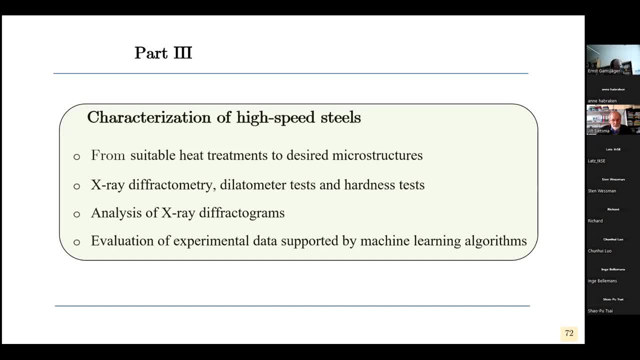 dilatometer tests and hardness tests And the X-ray diffractograms are analyzed, And then the evaluation of the experimental data are supported by machine learning, And then the evaluation of the experimental data are supported by machine learning, And then the evaluation of the experimental data are supported by machine learning. 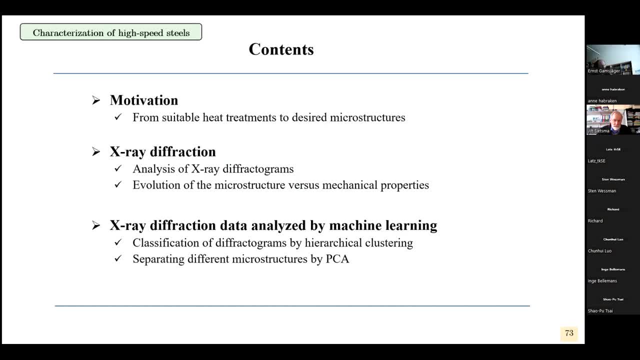 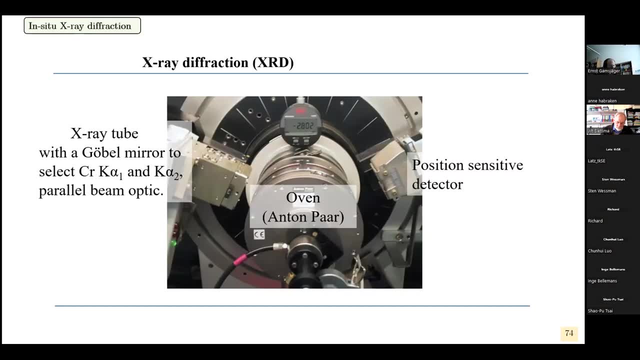 learning algorithms as the motivation. yeah, we want to come from suitable heat treatments to desired microstructures, and so i show you the experimental setup. this is uh, to measure the x-ray, x-ray diffractograms. here we have a x-ray tube with a goebel mirror. 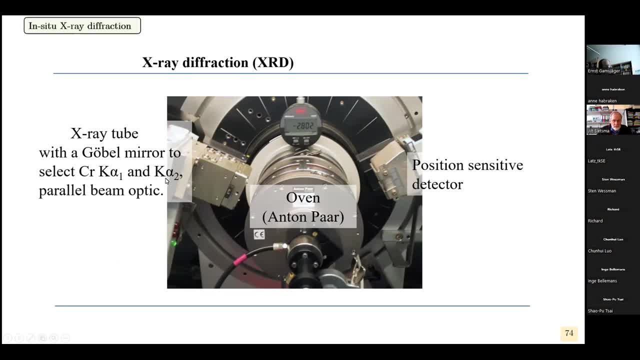 and we can select the chrome car for one and car for two with a parallel beam optic. here is the htk 1200 oven by anton bar and here we have, here we have- a position sensitive detector. and so this is how a typical diffractor 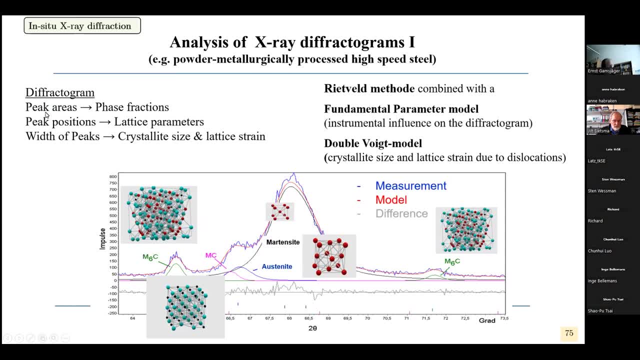 looks like and we can analyze the peak areas and from that we get the phase fractions and the peak positions tell us the lattice parameters and with the width of the peaks we can see the influence of crystallite size and the lattice strain. and in order to analyze this, 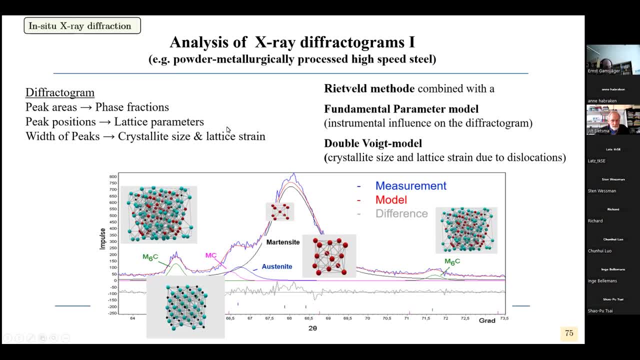 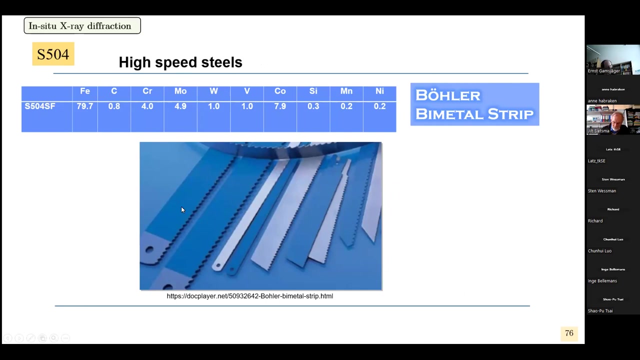 diffractograms, usually one vimosfriedfeld method emphasis dedicate. now i am demonstrating forces and narrows of the. When treated, when heat treated in a good way, one gets very, very good material properties and they can be used as a source, for example. 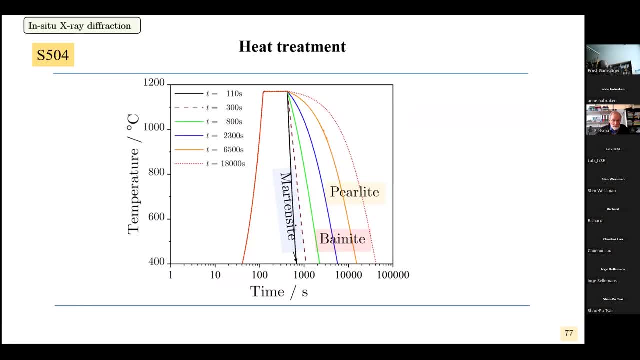 And here we look at different heat treatments. The time here is the T8. by 5 time means this is the time during cooling, when coming from 800 degrees Celsius to 500 degrees Celsius And you see, for very small times, 110, you. 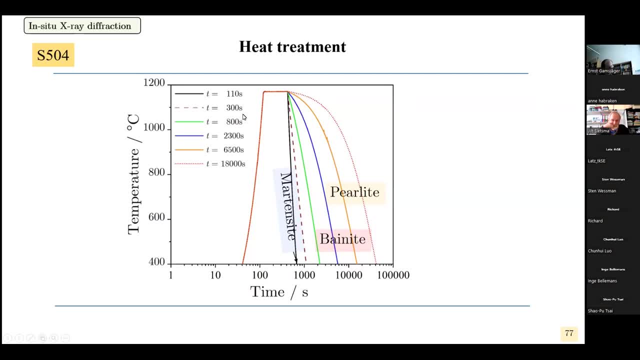 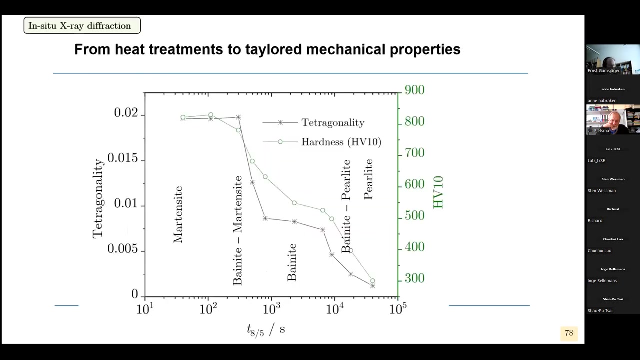 You get martensite and for 300 seconds also martensite, and then the amount of bainite is increased And for very small cooling rates and cooling times one gets finally the pearlitic structure, And here also from X-ray measurements. 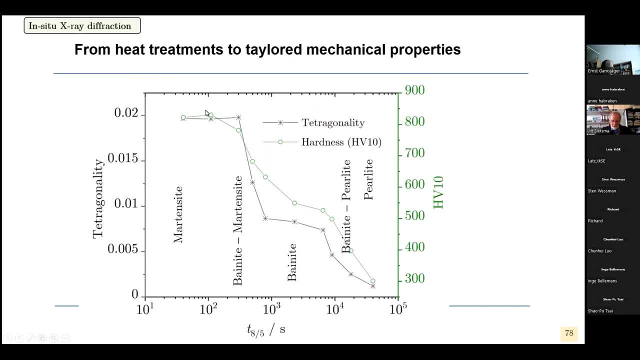 one can get the tetragonality which you see, for here is the tetragonality plotted versus the T8 by 5 time. And you see, for martensite there is a high tetragonality and then it goes down for bainite and martensite. 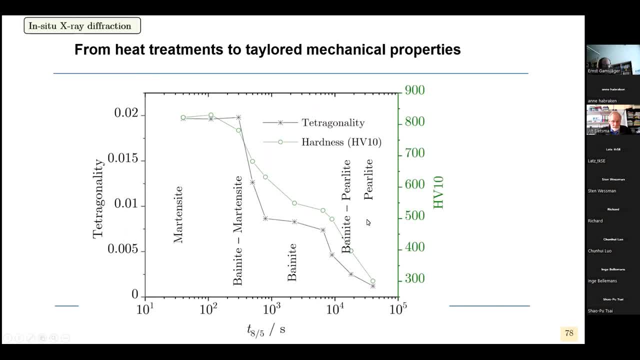 And it goes even down for when pearlite comes into play. And a similar trend And it goes even down for bainite and martensite, And it goes even down for when pearlite comes into play And it has the hardness which is plotted on this scale. 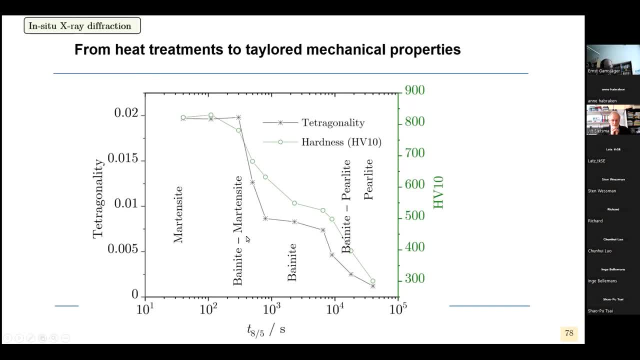 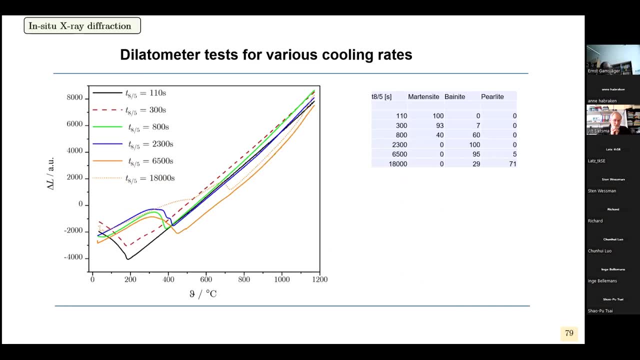 So it also goes down from martensite to bainite and martensite mixtures down to pearlite, And we did also telato-meter measurements. You see, for 110 seconds practically only martensite will come. You see here that the martensite Daddyyy argh. 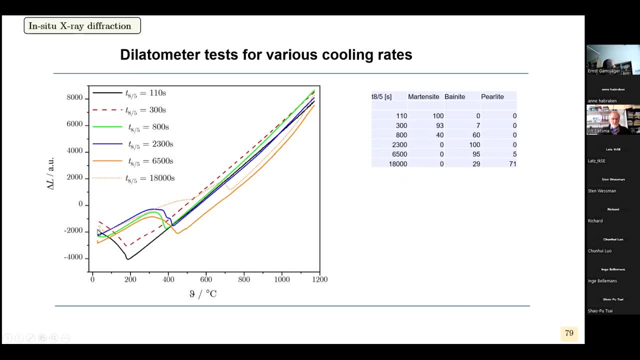 You see here that the martensite, the martensite appears, and for 300 seconds it's a martensite, but there is also a little bit of bainite, and then it's martensite. for 800 seconds we have bainite and then a little bit of martensite. 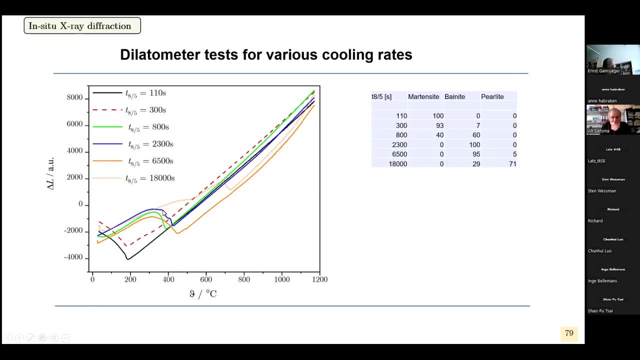 and then we have here upper bainite, lower bainite and almost no martensite, and for the very long cooling times we have here first perlite and here first perlite and then a little bit of bainite also. yeah, you can see the compositions and 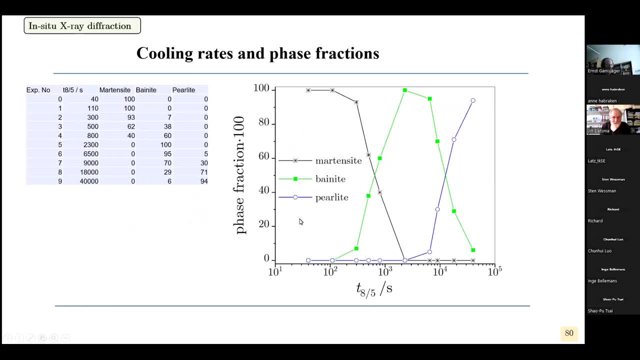 here. here is the phase fraction as a function of this cooling rate. we see it's a very long cooling time and it's very long cooling times. we have here first perlite, Again at high cooling rates. we have martensite, We have almost 100% bainite in the middle range of cooling. 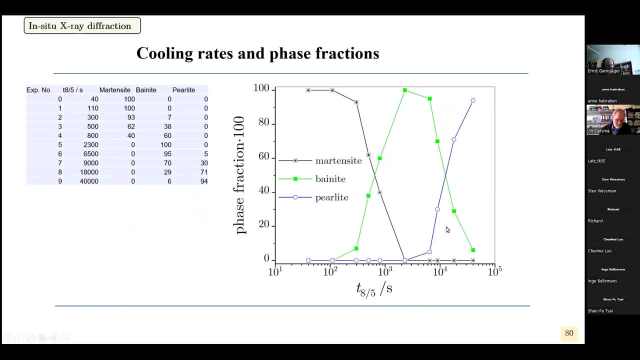 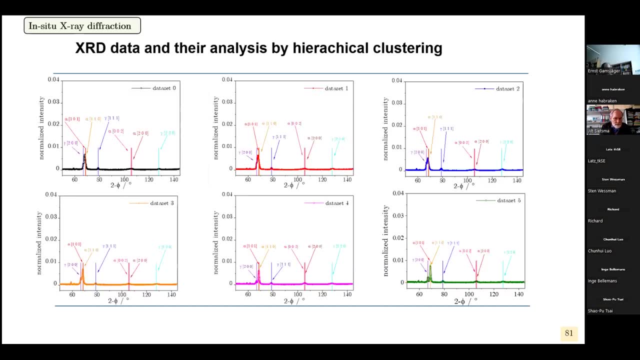 times And for the very low cooling times, the amount of perlite is increasing. And here are now 10 different data sets from the 10 different diffractograms here, starting with martensite and then going to perlite And, for example, here, when you look at the perlite here, 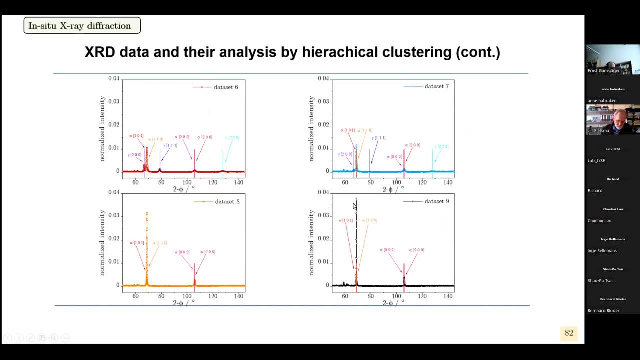 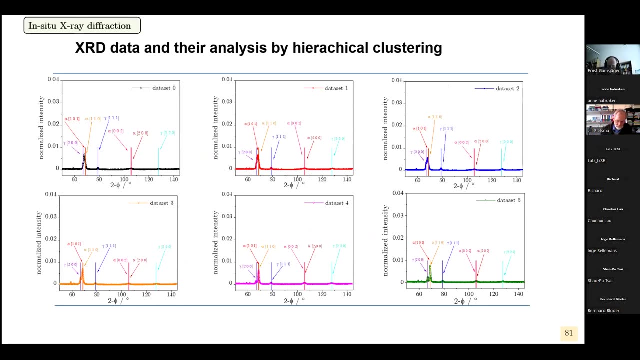 you get a very, very sharp high peak of the alpha- 1, 0. 1, 0. 1, 0. 1 peak, And it looks completely different here, And we know, of course, which data sets belongs. 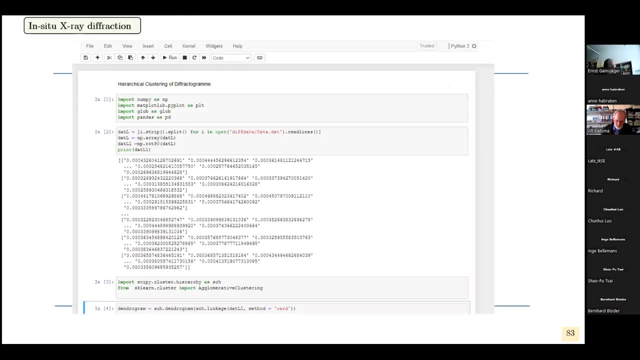 to which heat treatment. But now, with hierarchical clustering one can tell the machine the different diffractograms. here, All these 10 diffractograms are provided for these. This is a hierarchical clustering procedure, And a cluster means that the program 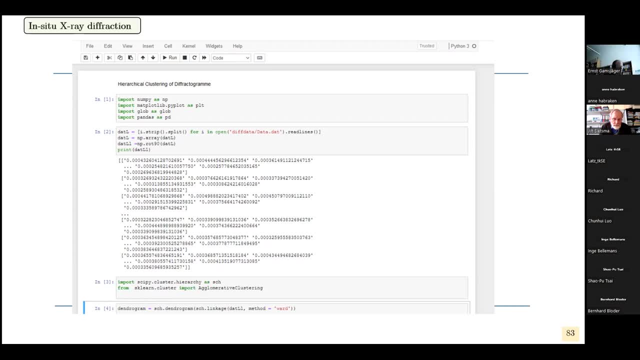 wants to sort to find different, similar groups, properties, And so first we have: all these diffractograms are one cluster, So we have first 10 clusters And then the program tries to put the closest clusters together. This is done here with the method of word.